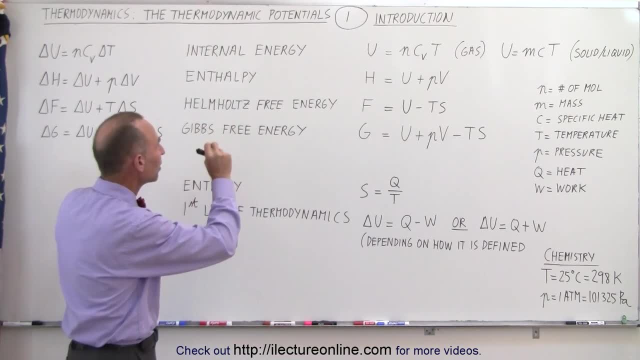 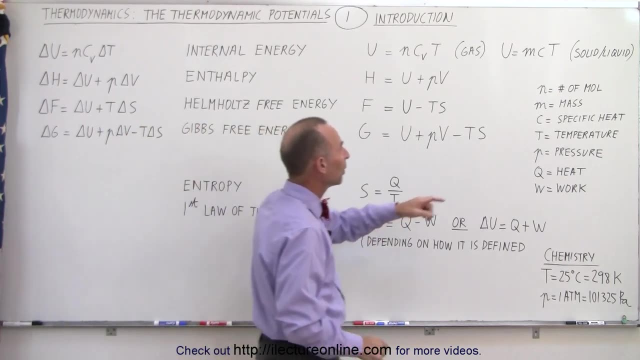 to go through these very systematically and explain what each one of these mean, with, of course, the necessary examples to make everything a little bit more clear as well. You have to keep in mind what these things mean. N stands for the number of moles. 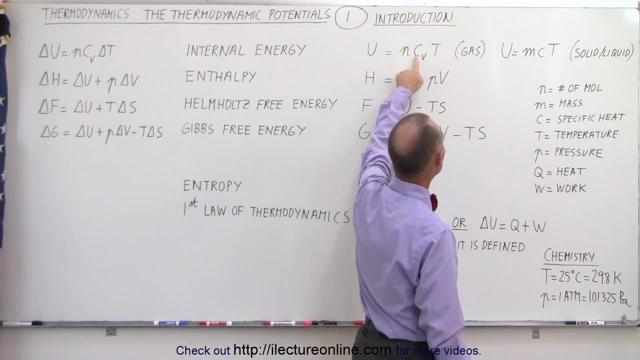 mass. C is the specific heat, C sub V is the specific heat at constant volume. Now, even though the volume doesn't remain constant, we still use this constant here to indicate the value for U, which is internal energy. if it's a gas, T stands for temperature. 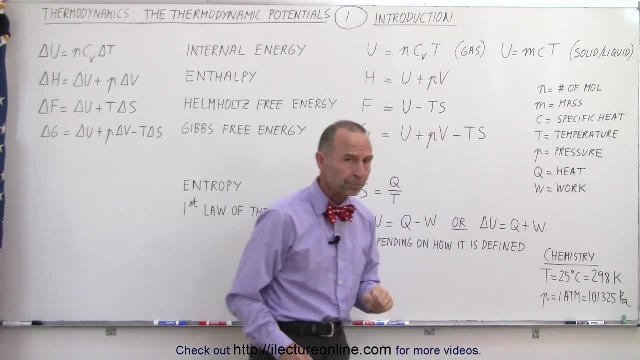 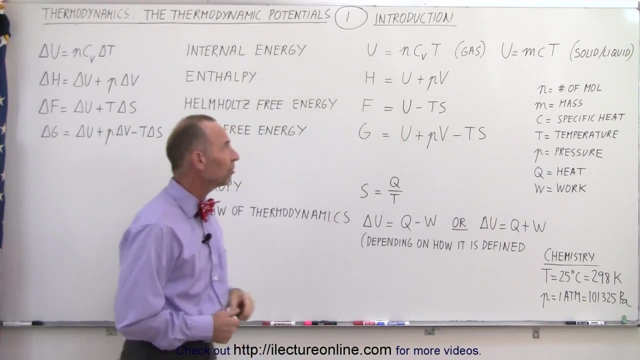 P for pressure, Q for heat and W for work. We're also going to talk a little bit about entropy because, as you can see, the value for S appears in at least two of the equations. so we need to know what that is. And entropy is defined as Q divided by T. And then, finally, 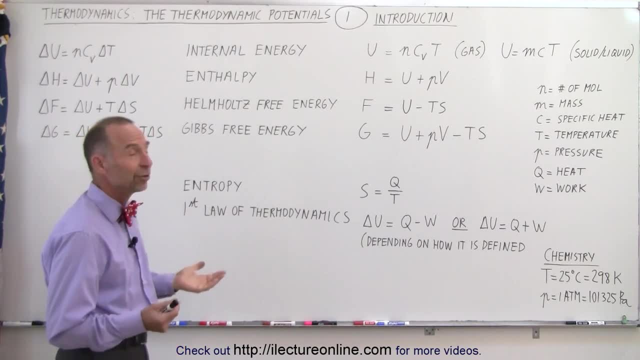 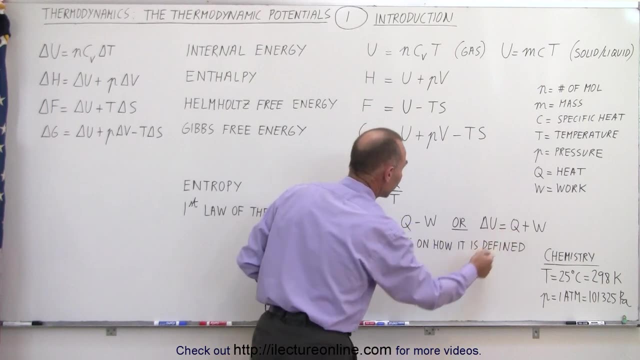 we also need to know the first law of thermodynamics, which is defined in two different ways. It's either defined as delta U equals Q minus W, or delta U is equal to Q plus W, And that depends how it's defined. Again, we're going to talk about that in more detail, But again, 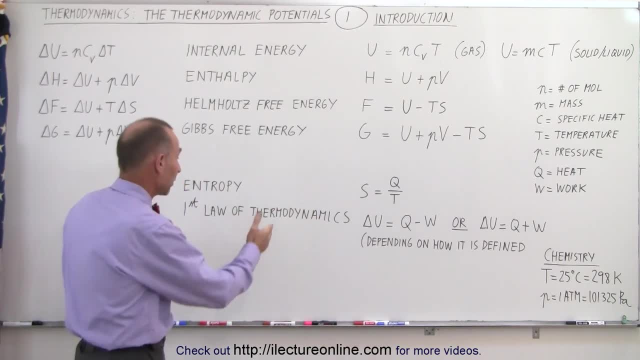 remember that delta U can be defined in different ways, depending upon which way it's defined, And then, of course, that's going to have a lot of difference. So let's go ahead and look at the other variables, called the thermodynamic potentials, Also, when we deal with these. 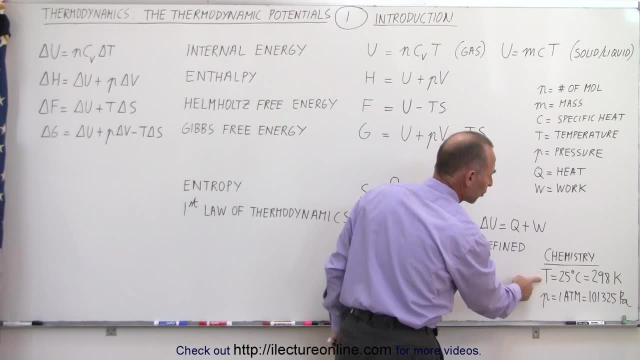 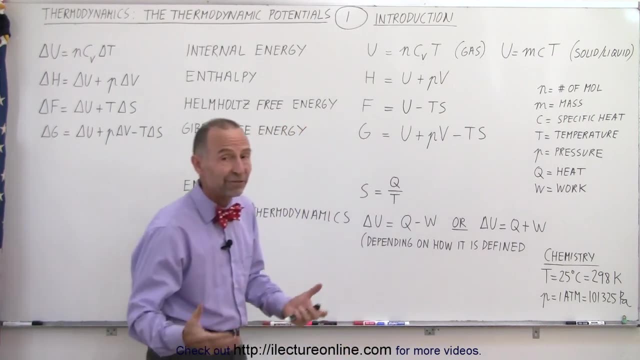 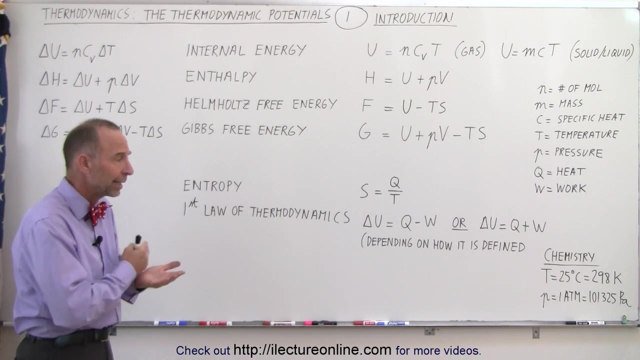 concepts. in chemistry, we typically leave the temperature at 25 degrees centigrade, or 298 Kelvin, and the pressure of one atmosphere which is 101,325 pascals. Now, that's not always the case, but keep in mind that during chemistry and when we have what we call chemical processes, 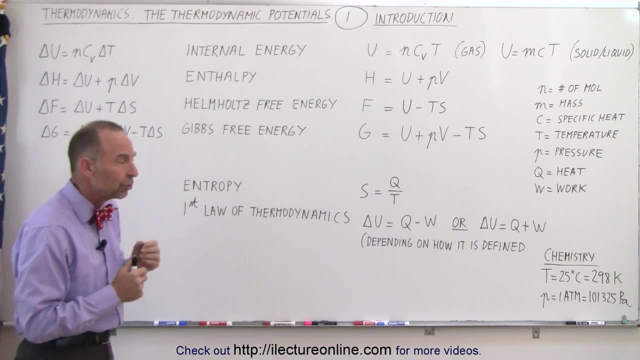 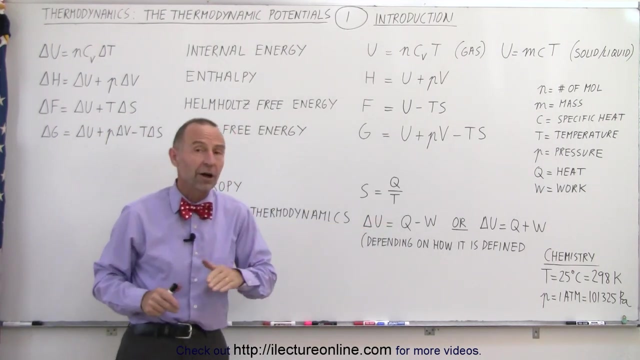 where heat is either absorbed or expelled. we typically do those under conditions, as we call the typical conditions, of 298 Kelvin and one atmosphere of pressure. So at this point we still don't know what that means. We still don't understand why there's a different definition of the first law of thermodynamics and how to. 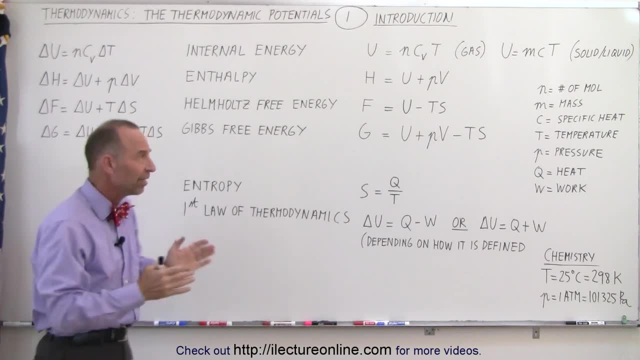 calculate any of these things that make sense out of them. But at least this is, in totality, what we're going to talk about in this section, in this series of videos, and we're going to take it very systematically to make sure that everything works out. So let's get started.